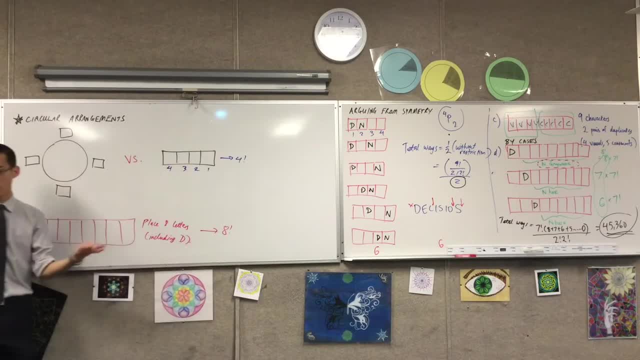 So that's why this becomes four factorial, N factorial, depending on N spots, No problems, okay. But but when you take the same four people right And you want to place them around a table, okay, There's one minor difference, okay. 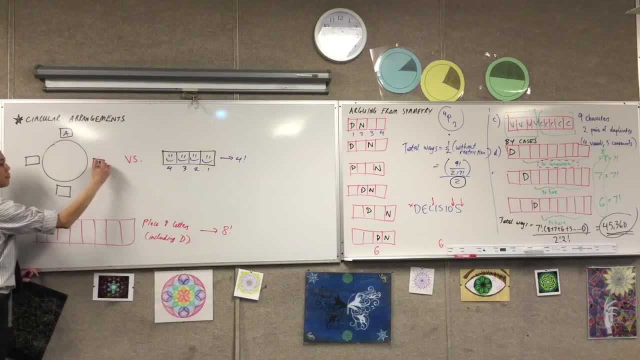 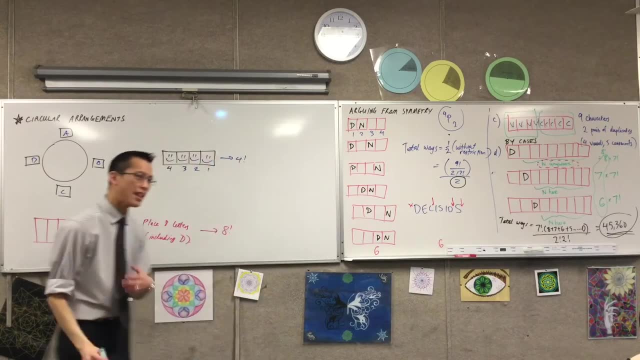 Which is that if you put, for instance, if you put A here and then B here, and then C here and then D here, okay, That's, that's one of the possible arrangements. Do you notice that had the first person- let's call them A- had they chosen to sit over here? right, But then suppose, like: 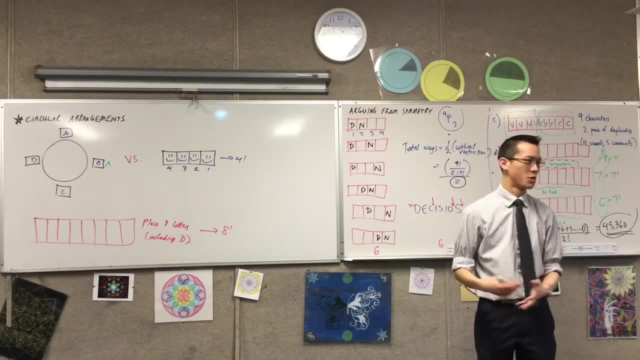 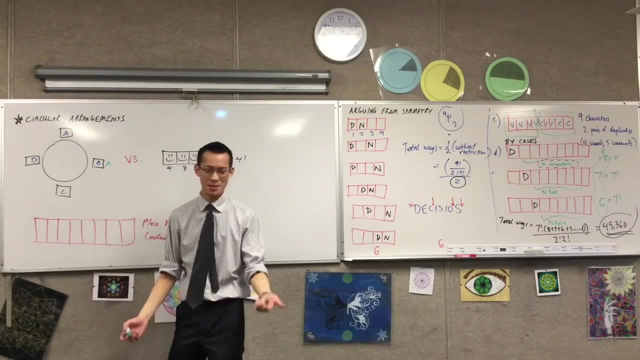 A's right-handed and it's like: okay, the next person who arrives is like: I don't want to sit on your right because you'll keep on bumping me into chopsticks or whatever. okay, So B the second person. hey, it happens right. 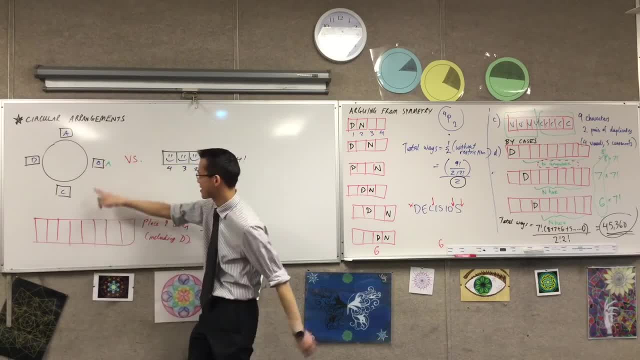 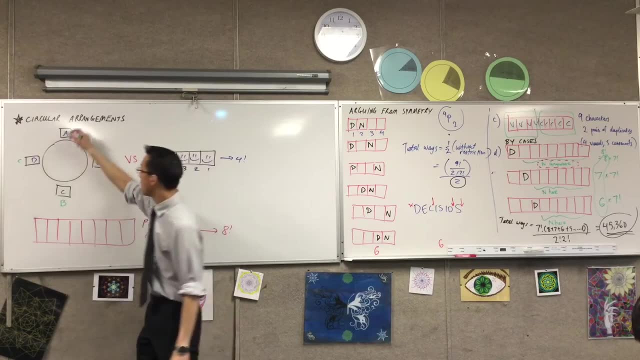 Two people in my family are left-handed, so we have lots of fun in situations like this. B is going to go to the left and, you know, suppose they're all right-handed, So then C will go to the left of him and then D will go to the left of him because they're like: ah well, there are no more spots left right. 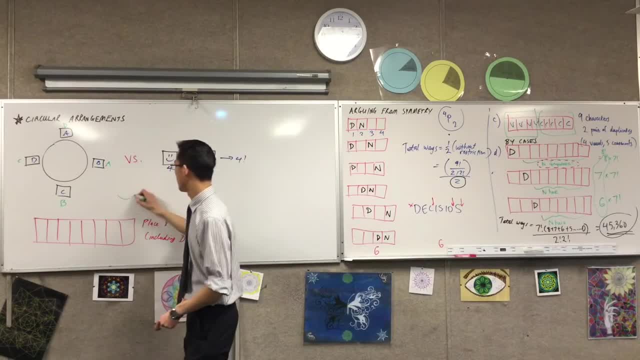 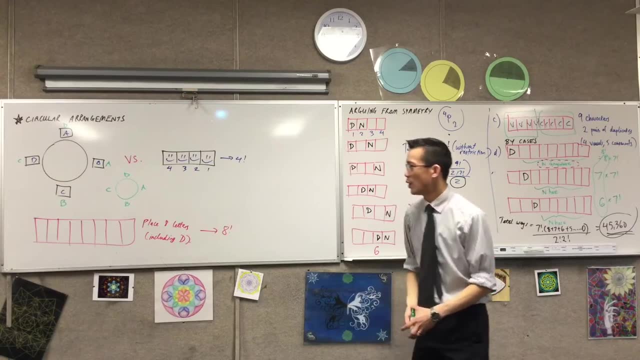 Now, when you have a look at this arrangement, let me just redraw it down here: This green arrangement and the blue one. they're the same arrangement. They are the exactly the same arrangement. If you were to ask each of the people, you know who's to your right. 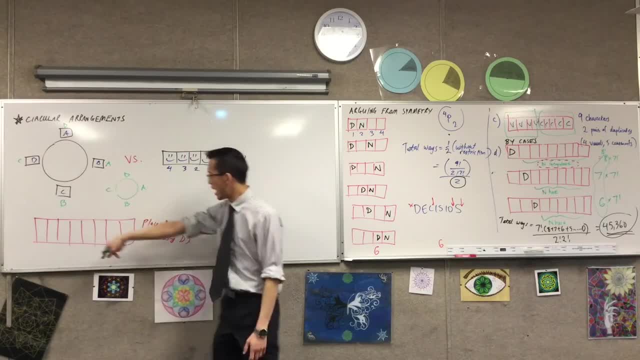 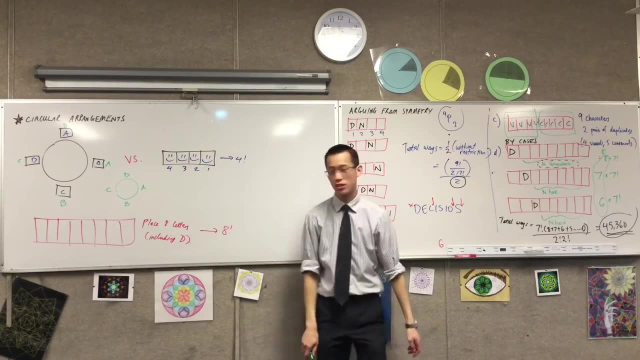 okay, If you ask them under this situation, they'll all give you an answer. and if you ask them in this situation, they will still give you the same answer. The same person is to my right every time. All you have to do is just turn your head 90 degrees to the right. 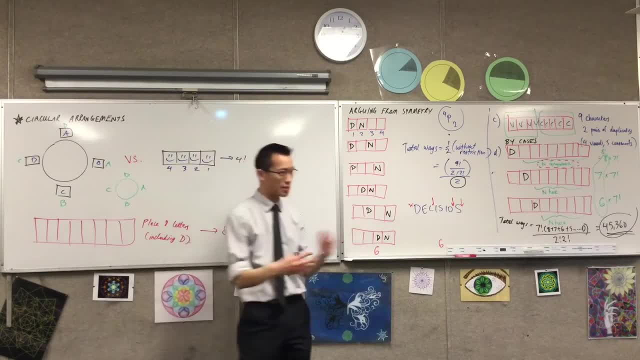 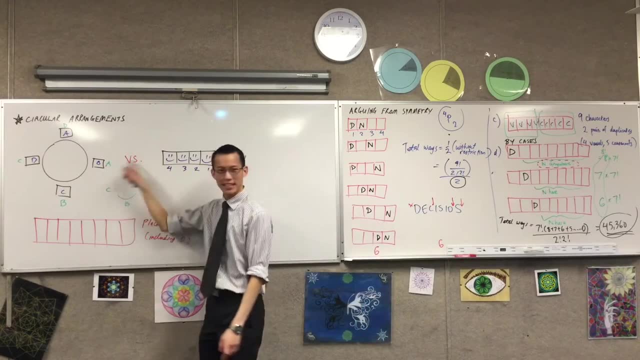 You know, there it is right: A, B, C, D, It's identical, okay. So what you've done is you have over-counted. How many different ways can I keep on spinning this table around and have the same arrangement? And the answer is four ways, okay. 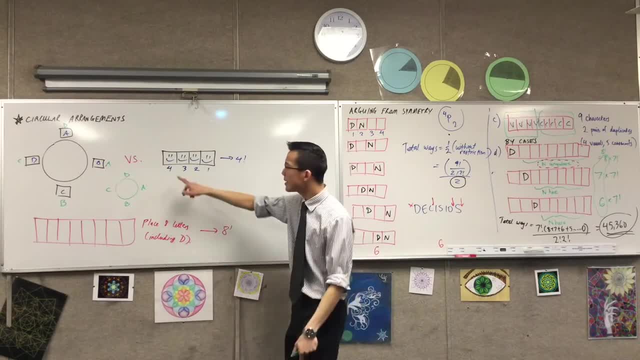 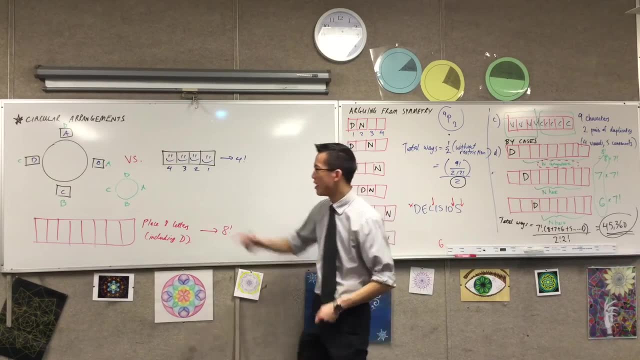 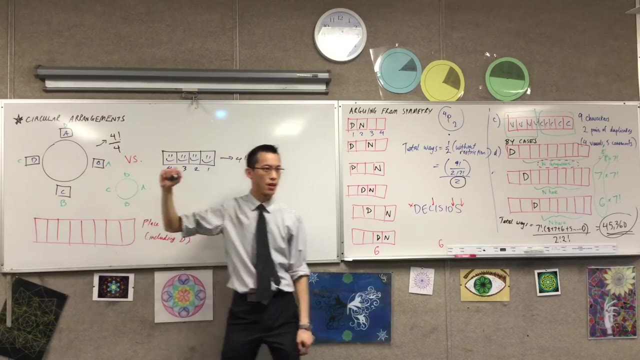 So I can think about this in two approaches, right? I can say four factorial is fine, right, But you've always over-counted by however many chairs you've got, right. So this is therefore not going to be four factorial, It'll be four factorial. and I'm over-counting by how many seats I have, right, Because I can keep shifting them around. 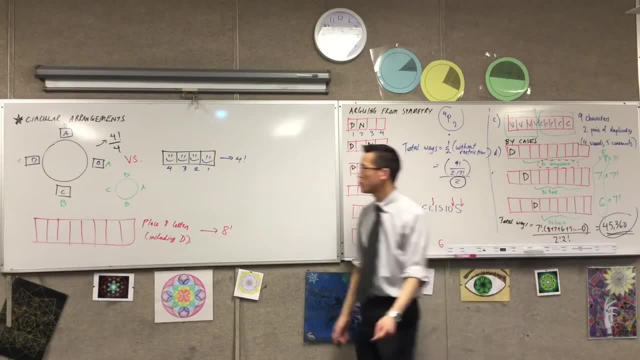 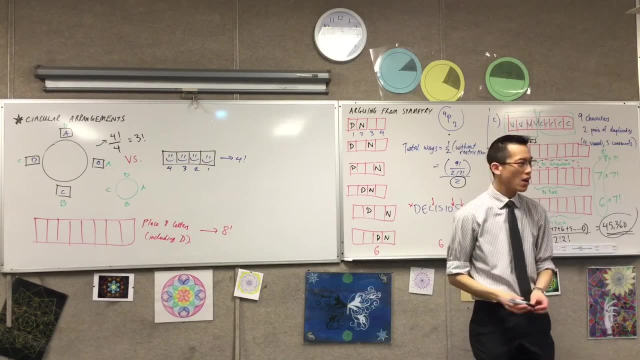 However, then you'll notice, right in the same way that we did here, you're like: well, that's just going to be three factorial. Instead of n factorial, it'd be n. take away one factorial. Now, why would that be? 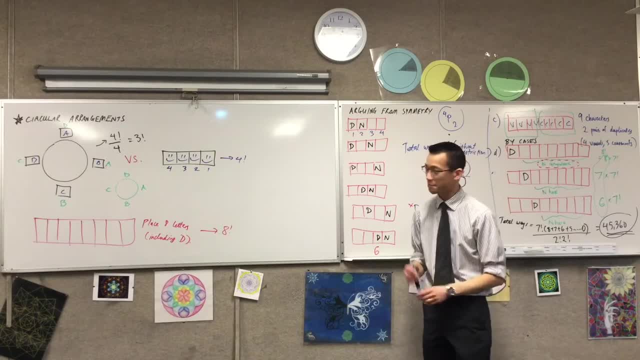 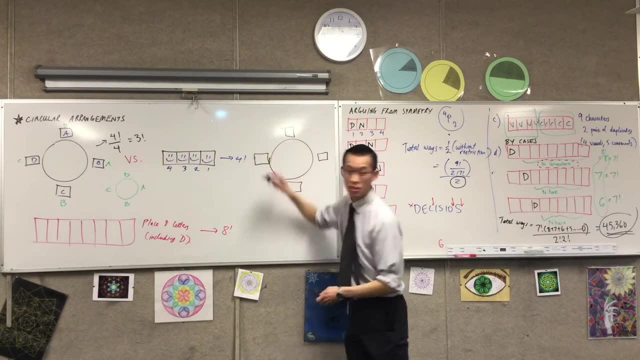 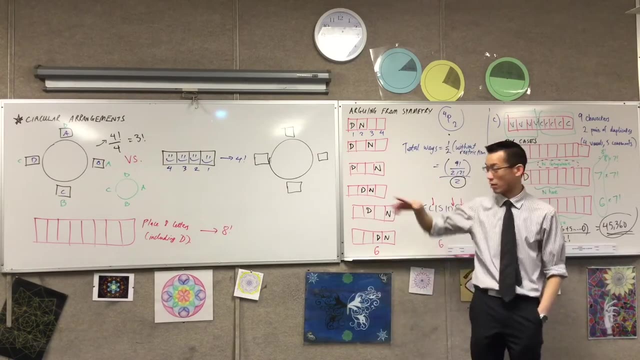 How can that unlock a helpful way to think about this? okay, Think about this again When you're the first person right. So you arrive and you look at this setup. okay, Now, when you look at this- all of the tables, sorry, all of the chairs around there- they look identical to you, don't they? 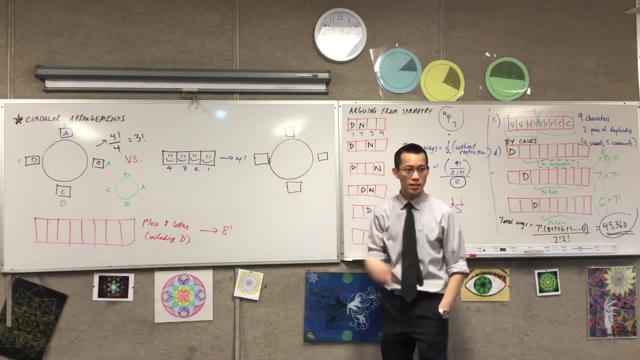 Like sitting here to sitting here, to sitting here to sitting here doesn't make a difference to you, right? They're all the same. There's no people to say, oh, who's on my left or who's on my right? okay? 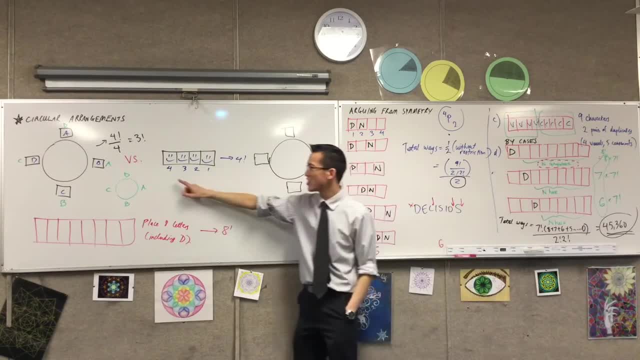 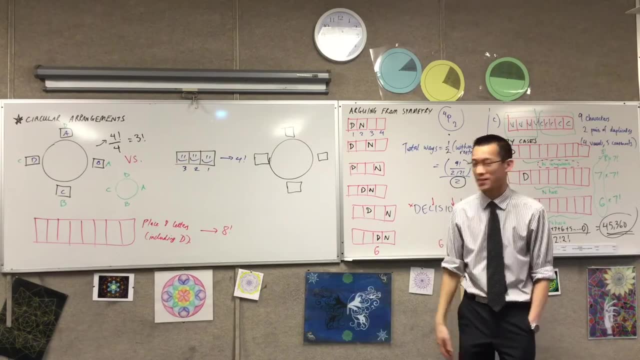 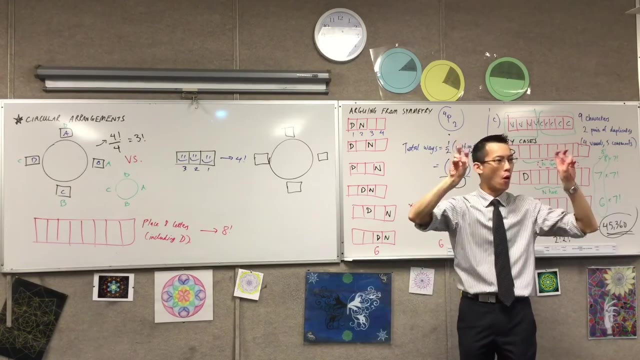 So therefore, this first person actually contributes. they don't contribute any extra choices, right? The first person doesn't really have a choice because all the choices are identical, right? I guess another way of phrasing that is, there is inverted commas. one place to sit, which is: 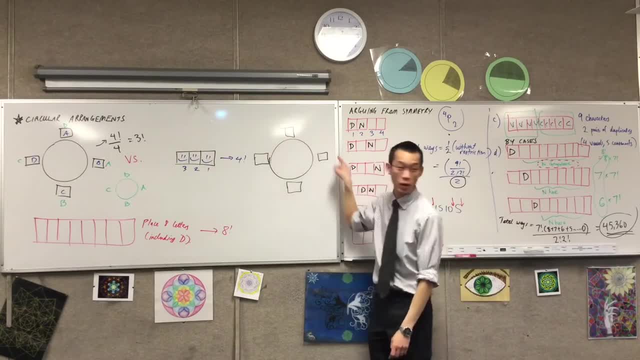 anywhere, okay, They're all the same. If it was here, here, here or here, it's like: well, this set of cutlery looks the same, and the same person who's on the left is on my right. 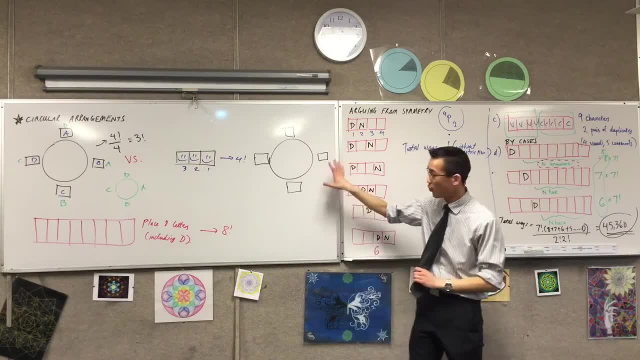 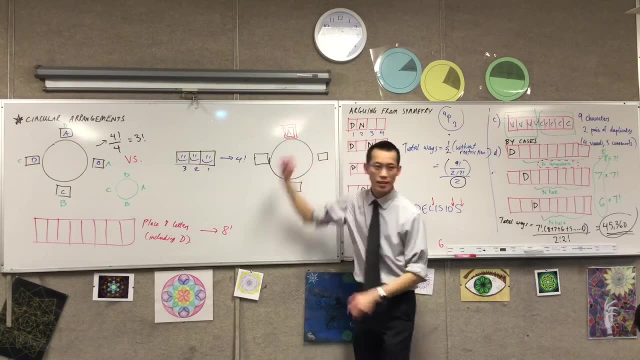 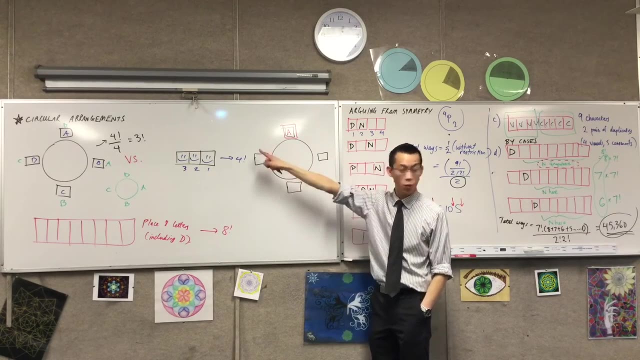 you know, I'm in Club Lonesville, right? So therefore the first person contributes nothing, right? But once he sits down or she sits down, this then becomes the same as our normal problem, right? These positions three and then two, and then one. 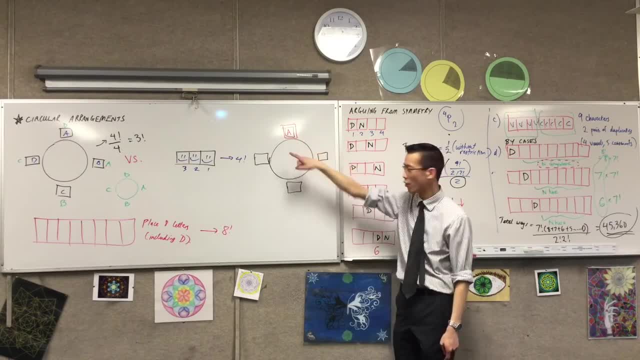 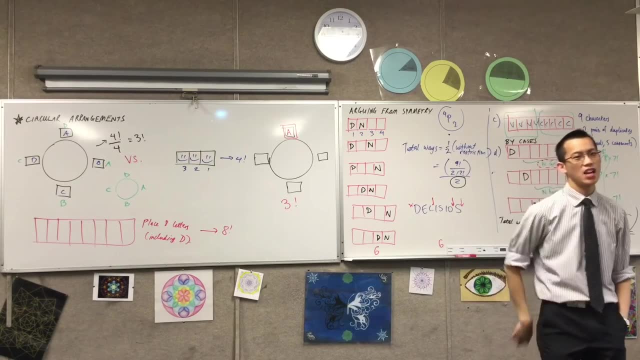 they have an order to them, because you're either going to be on A's left or A's right, or opposite A right. So therefore, this is just three positions to fill in any particular way. That's why it's n take away one factorial, okay. 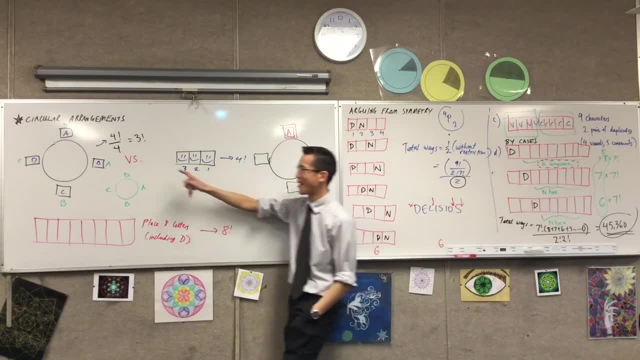 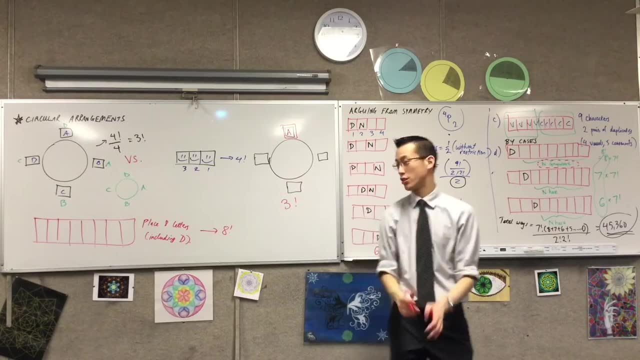 So all this comes down to is, when you see circles, right, Just make sure you're not thinking of n. you're thinking of n. take away one and then treat all of your conditions and restrictions in exactly the same way that we've already been doing, okay. 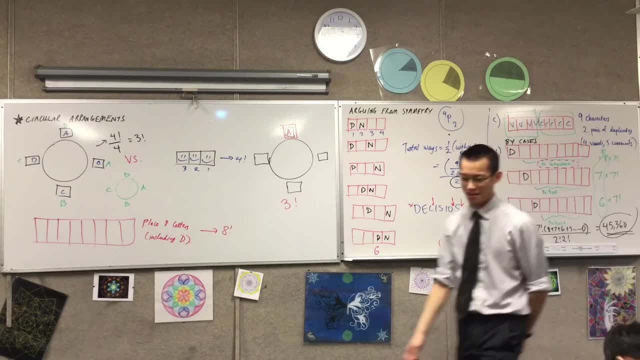 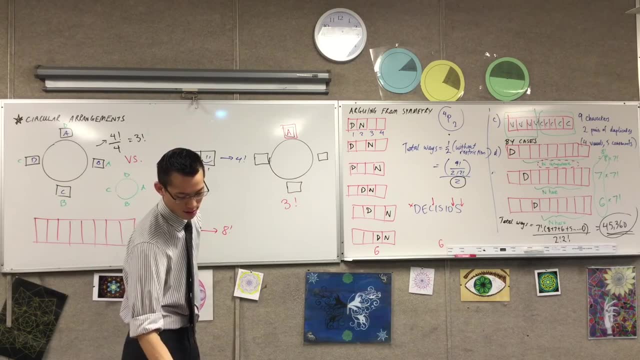 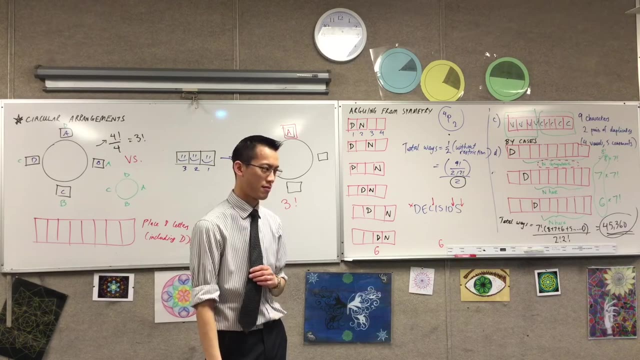 Any questions? Right, yeah, In instances where, for a circular motion, there might be a question where it's like a specific case where it would actually turn out to be like trying to arrange people in a straight line. Did you say circular motion? 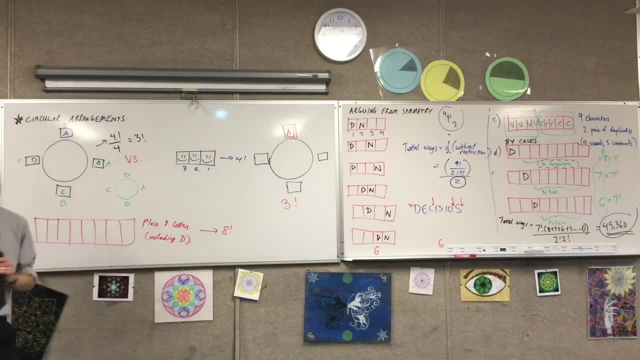 Yeah, Ha ha ha, Arranged Um, yeah, yes, yes, So, um, what you need to do is pay careful attention to the restrictions you're given, okay, So, for instance, this exact one that I mentioned, right? 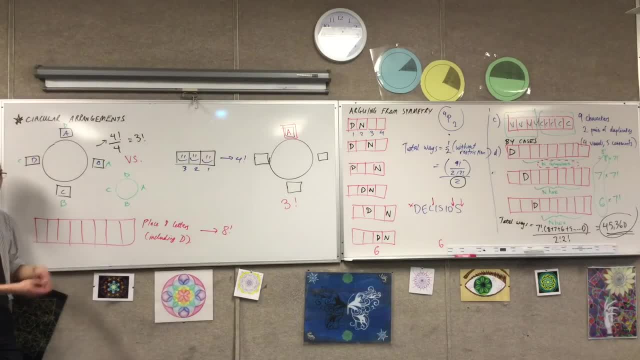 Like, oh, um, you know, Mr Wu doesn't want to sit to the left of his brother because his brother is left-handed, okay, Which is exactly how I've lived my life, okay. Therefore, therefore, what you would do is you would fix my brother in a spot and then you work out the rest of these guys and you just say: I can't sit there, alright. 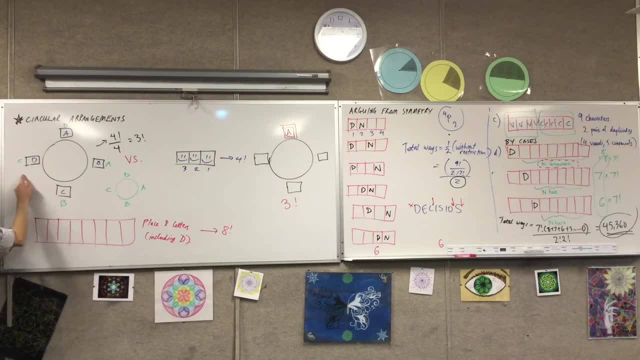 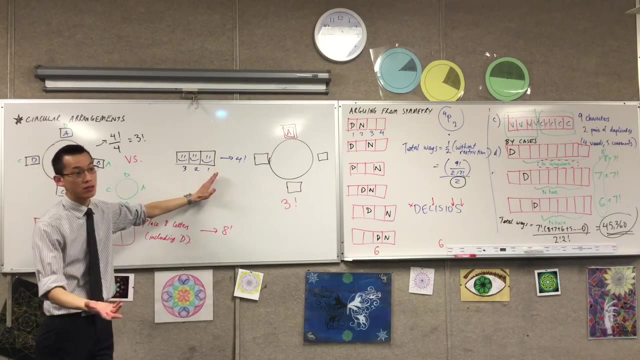 So you'd say, well, I've got two to choose from, and then you fill the others in two factorial ways, okay. So in some way, though, you've got to turn this from a circular right, where the positions don't matter, where it's like sit wherever you're lying, to something where it's like, okay, this and then this, and then this, they're my restrictions, okay. 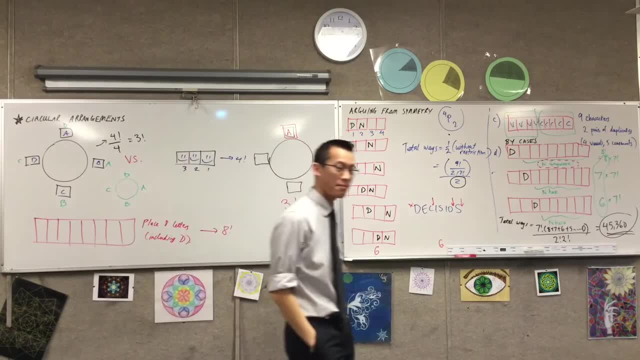 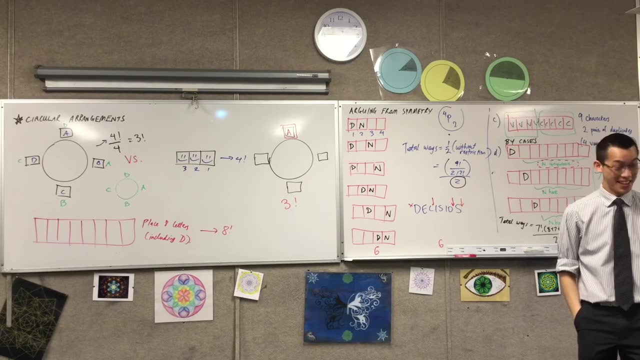 Yep, Ms Bell also talked about like necklaces and bracelets and how you can flip them over and stuff Like are we going to do that? Yeah, yeah, Are we going to do that. Um, I've sort of already taken that into account here. 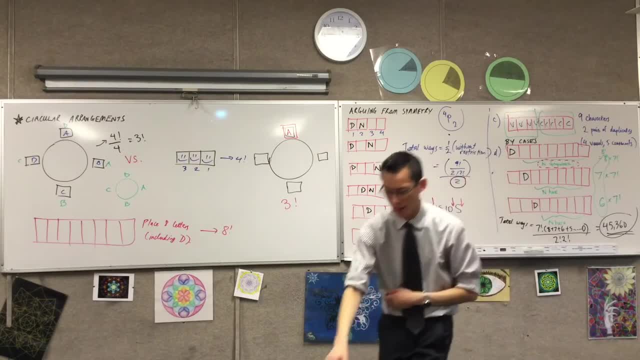 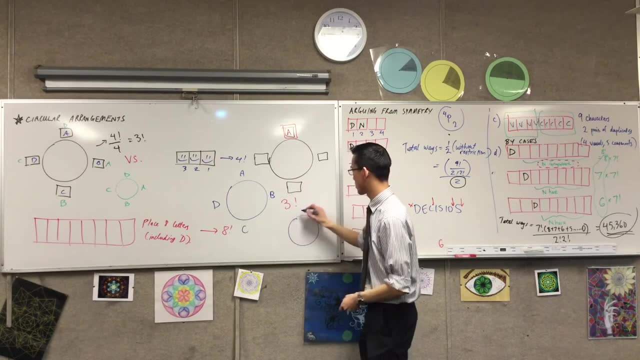 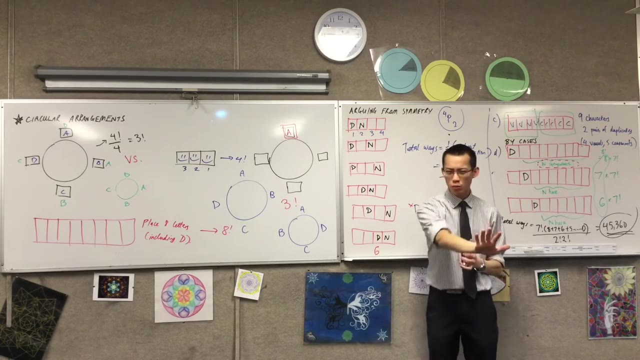 When you talk about flipping something over, okay, so they're thinking about this Versus this, Okay, So I've flipped these over, okay, Now I wouldn't worry too much about the way that was just mentioned, because when you have a look at these, are they the same. 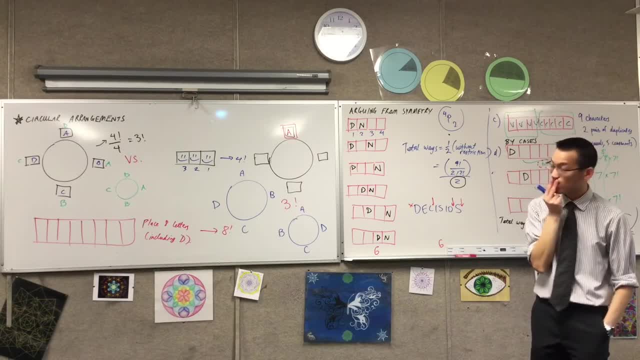 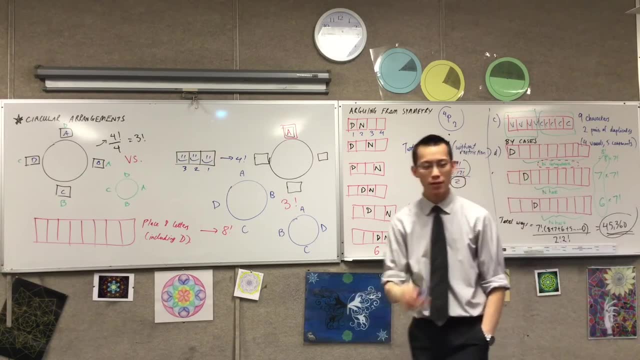 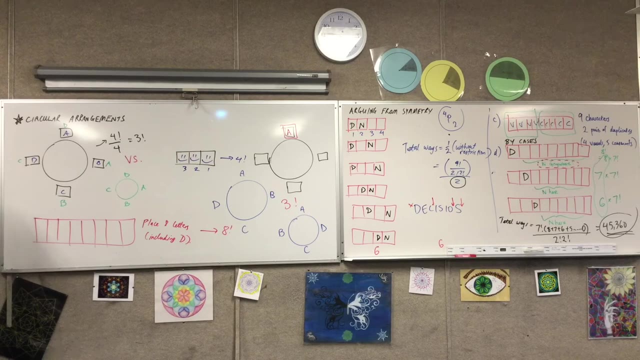 No, Yes, No, in some ways, No, Oh, Oh. Hmm, It's the same bracelet, So I'm going to repeat that original question I said to you, right, which is that if I asked all of these people who's on your left right, are you going to give me the same answer for one versus the other? 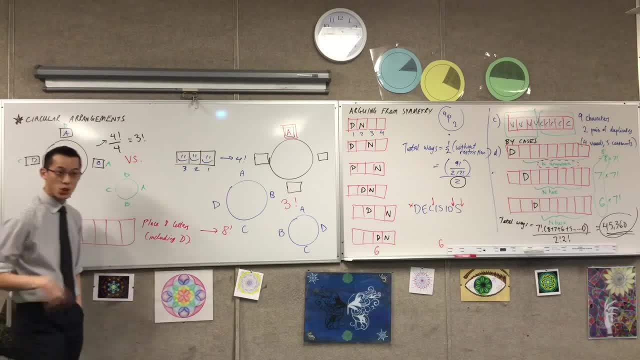 No, And the answer is no, you're not. So this is a different arrangement, right? This could make the difference between me butting elbows with my brother all dinner like- and for a Chinese beggar it's like three hours right- versus having a really lovely evening. 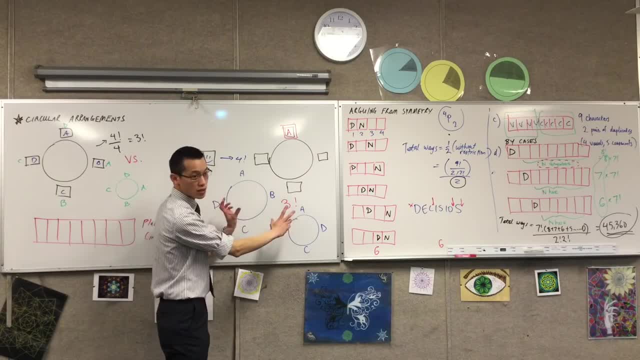 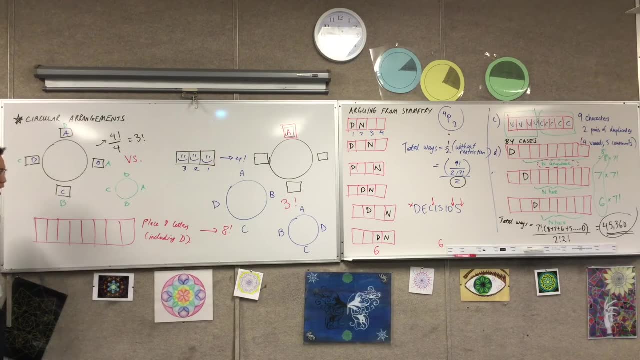 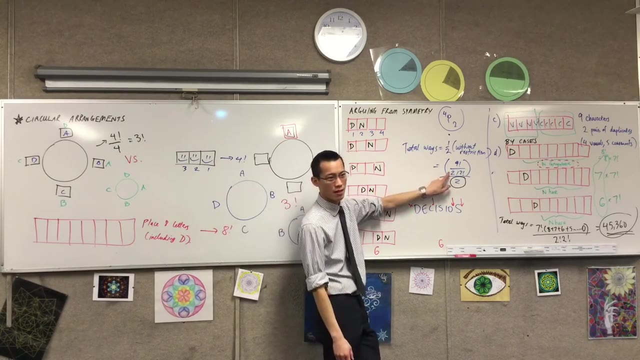 These are not the same arrangement, okay, So you can't just flip over. These are different permutations, so I can think of them as like all that matters. Don't worry about that, Okay, Okay, Where you would start to worry about that is if you have like a series of identical elements. but we already know how to deal with identical elements, right?